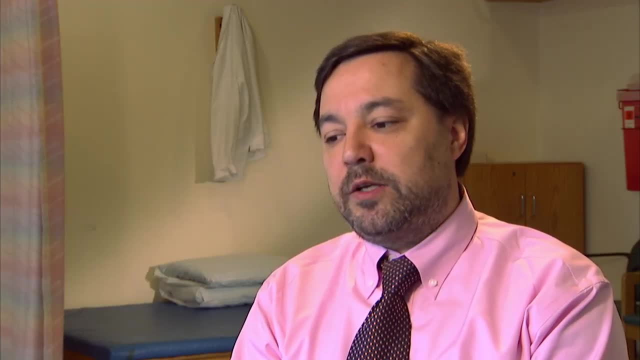 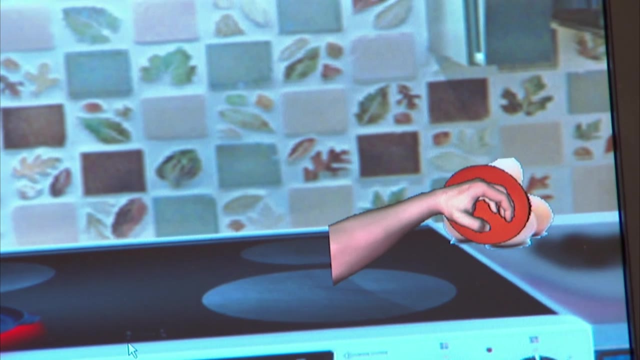 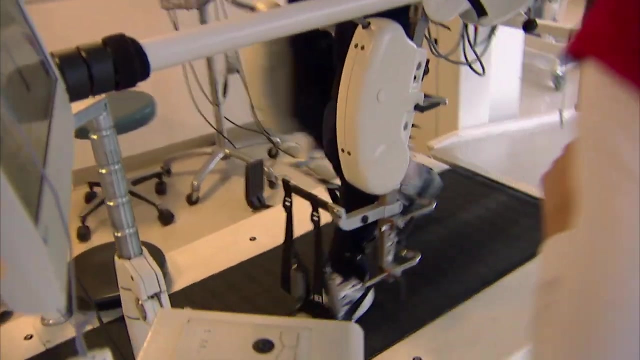 A major question that we're trying to address is whether, through the interaction with a robot, a person can actually learn motor tasks. That's essential in stroke survivors, in traumatic and injury survivors. The Locomat is a robotic exoskeleton for robotic gait training. 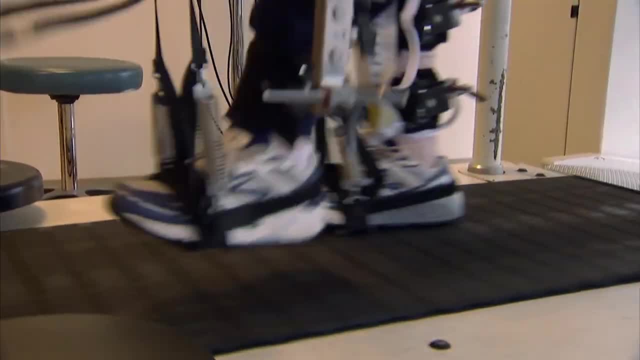 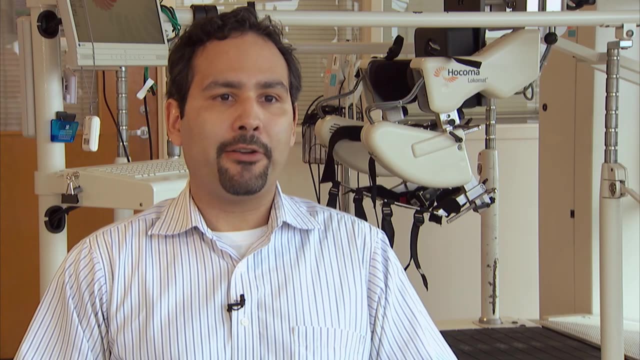 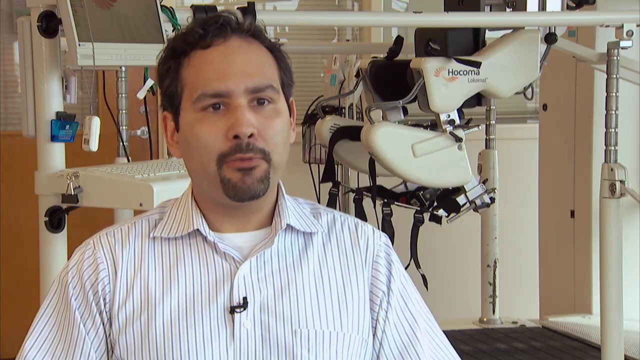 We'll make you walk a little bit faster now, okay, Okay, Okay, Very cool. Manual gait training, as was usually done, was really strenuous on therapists where they had to independently move the person's legs through the standard walking pattern. 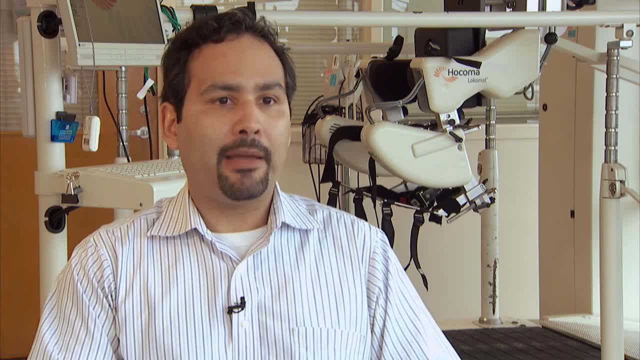 I want you to think about pulling your knee up and then you put your leg high and then you take this big, giant step. We've formed a collaboration with of the company that developed the Locomat, and so we're actually able to tap in, using our own software, and change the way that. 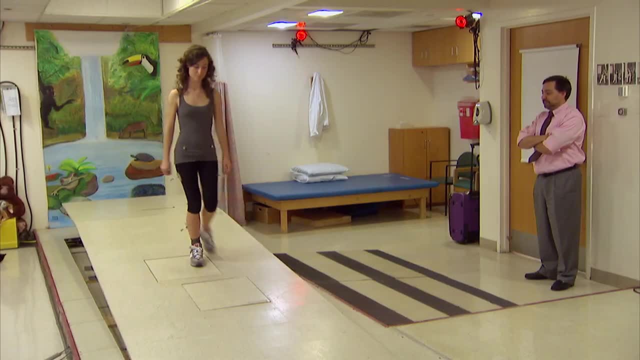 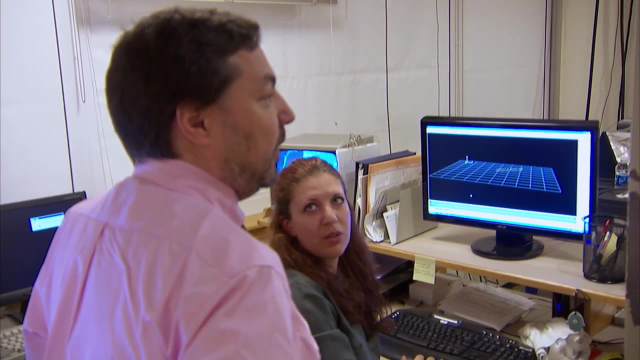 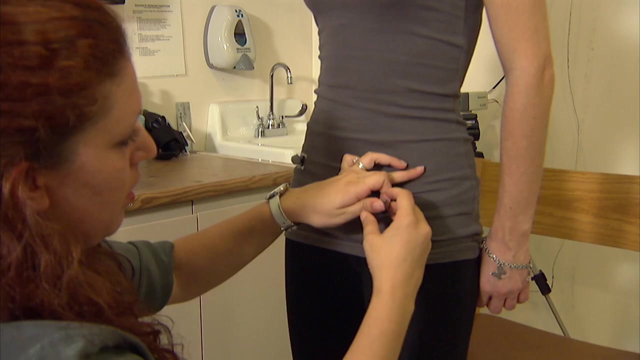 the robot works. The Marsh Analysis Laboratory was established to perform clinical evaluations, mostly in children with calc, tv cerebral palsy. We have eight infrared cameras that go around the room and point in the central walkway. The cameras emit the light that gets reflected from the markers and the computer can pick. 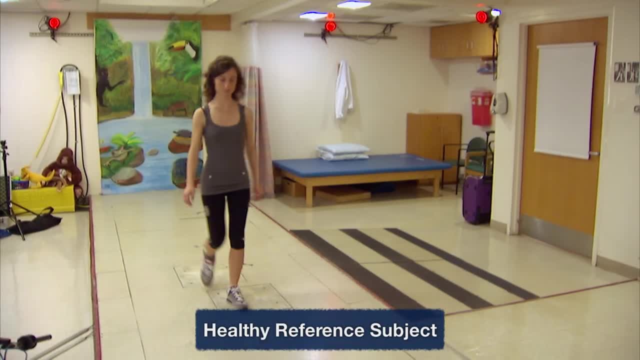 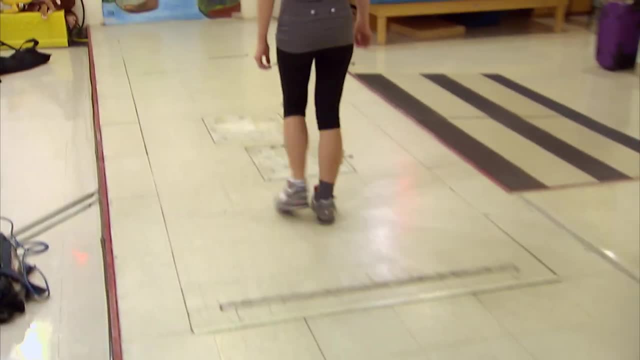 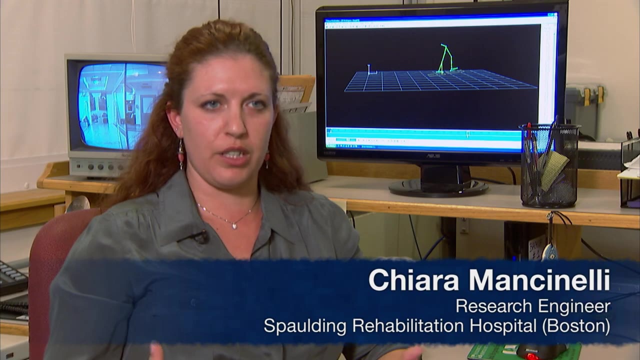 up the movement of the markers. The green lines show the different body segments, while the yellow line represents the force that is exerted during gait. That's something that will help the doctors in seeing how the outcome of surgeries or intervention lasts through the time. 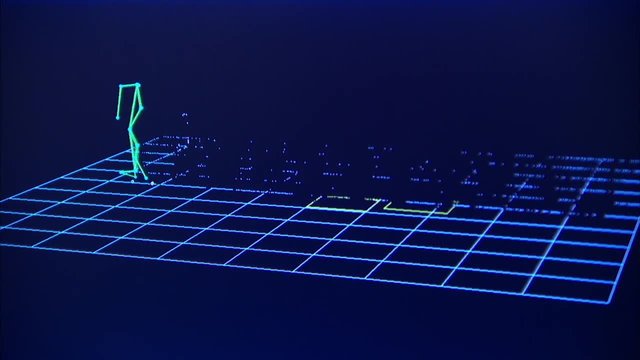 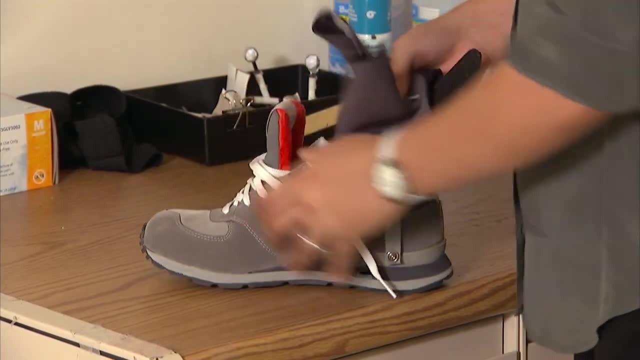 A lot of times when they come in, they want to impress the clinician, so they tend to walk better than what they would do when they're at home. The shoe that we have developed has sensors that are embedded in the sole of the shoe itself. 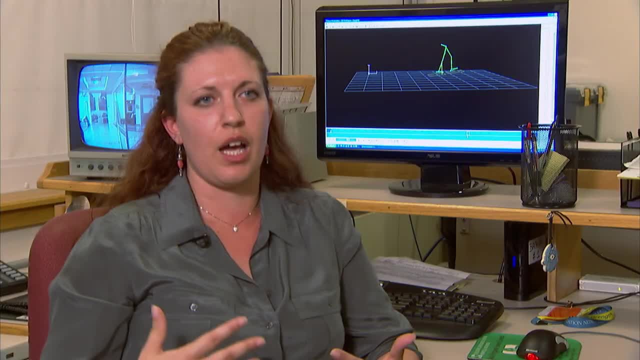 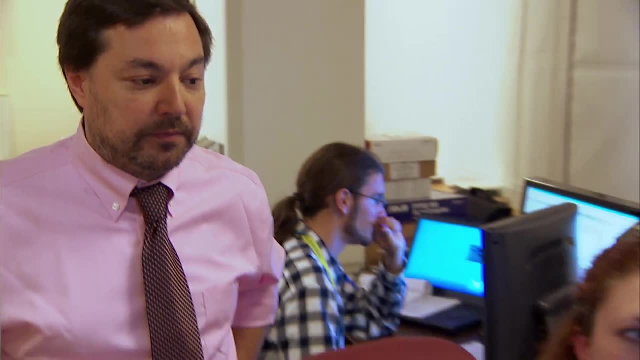 Once they put the shoe on, it's like wearing a normal sneaker. You can have monitoring that is less obtrusive And it's conducted in the same way In their home environment. so we can actually collect more data and have a better insight. 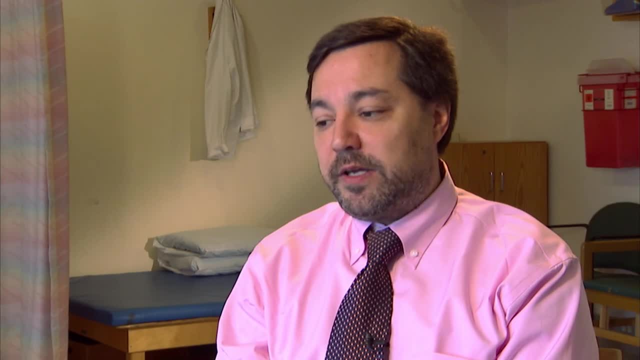 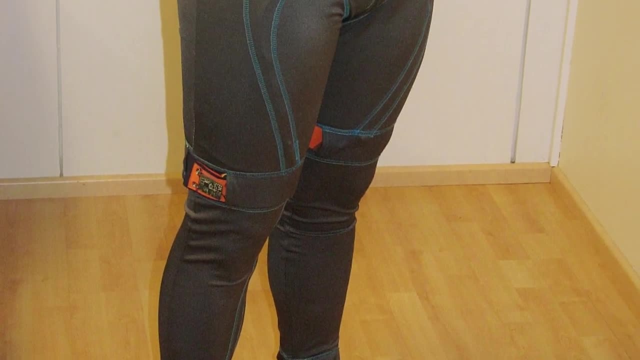 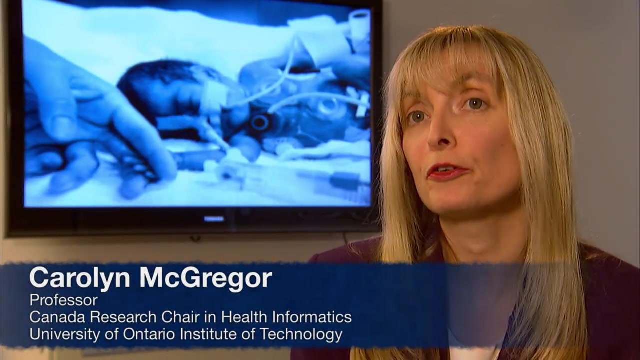 on how the disease progresses. Wearable technology has become possible over the past ten years because of major developments that allow us to integrate sensors into garments. We have the potential that if you can wear some form of a monitoring device, that your vitals can be monitored on a more regular basis and we can send that information through. 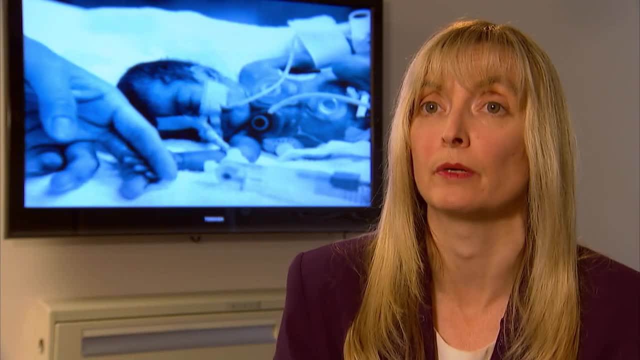 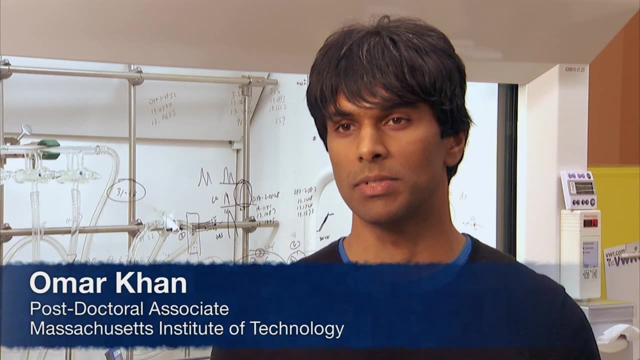 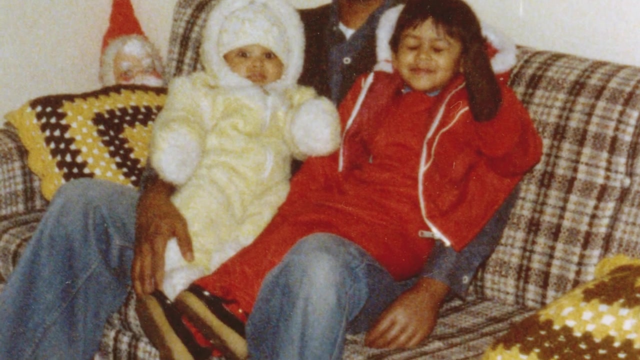 a cloud environment Before you need to go into an emergency department because you're very unwell. My father is actually an amputee and when I was young, I promised him I'd make him an arm one day. An amputee can live their life pretty normally with a prosthetic, but the idea that you can 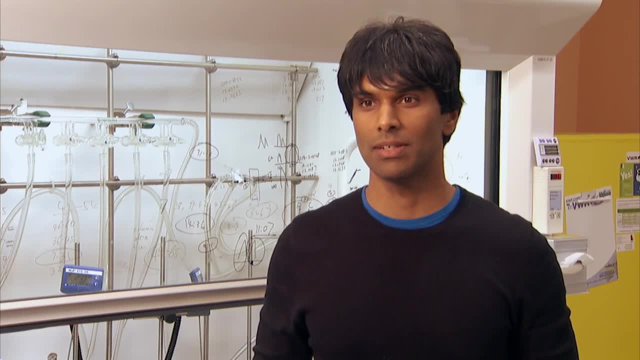 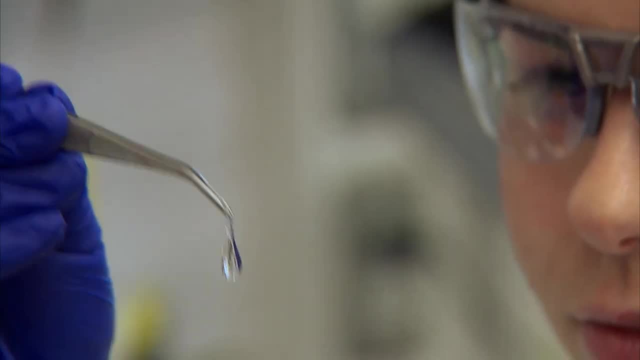 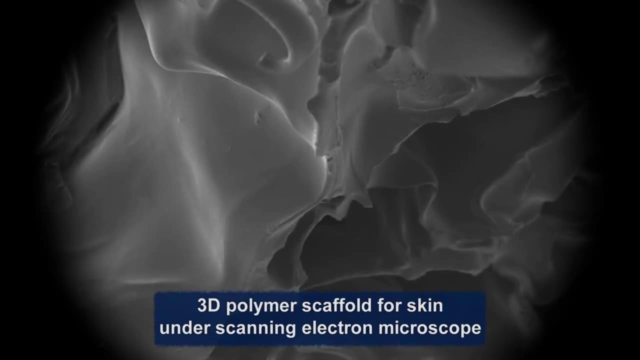 just take it to that next level. that's important to me. One way to do it that we've developed is you can take a plastic scaffold, a polymer scaffold. That could be whatever shape you want, depending on the organ or tissue you're trying to make. 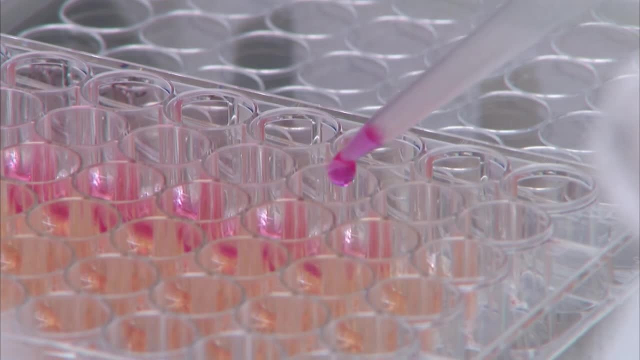 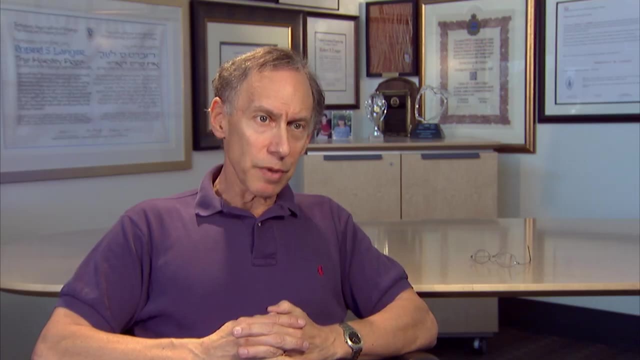 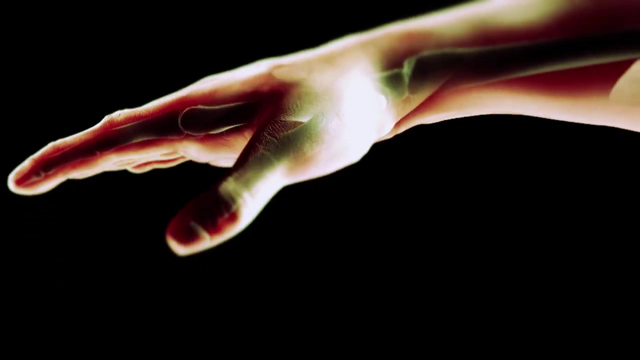 Then you might put certain cells on it and give it the right nutrients and also the right mechanical forces, grow it to a certain point and then do a transplant that onto the patient or into the patient. If you think about how complex the organ is, it's really difficult to mimic what happens. 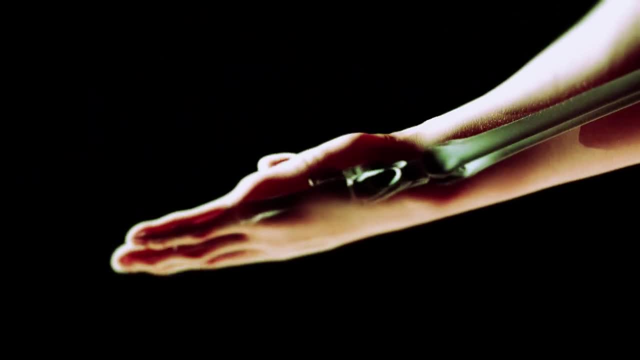 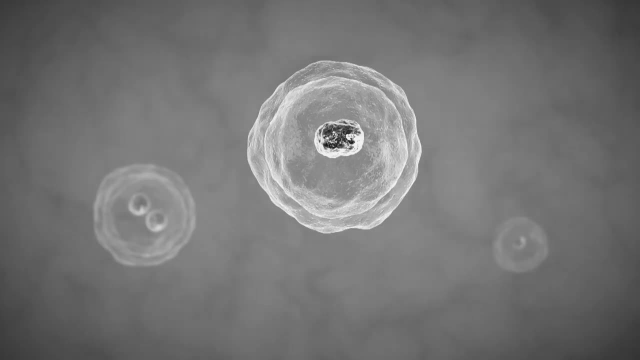 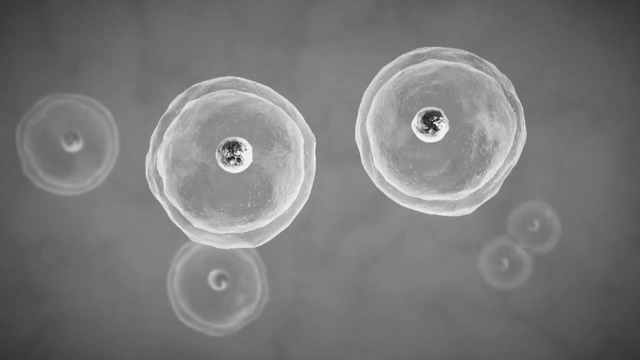 in nature. One of the big challenges is the vascularization. Also, in terms of stem cells, they are a long way to go. We have to understand what makes them differentiate. How can we control them so that they will not develop cancer? We're working on making various tissues and organs in the body. 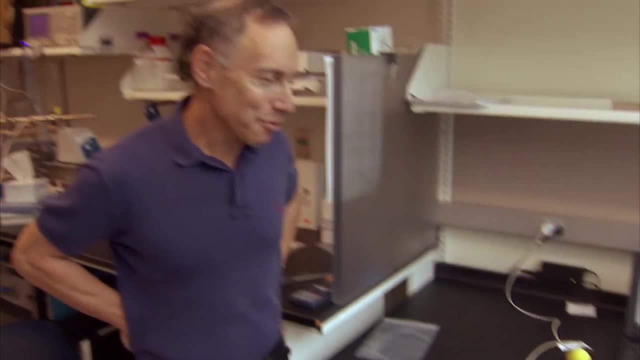 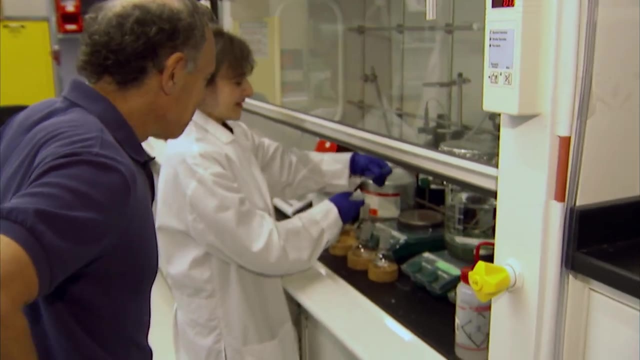 I mean new spinal cords, vocal cords, new intestine heart tissue, so there's a whole range of things that we've been working on. How are the micro-bubbles Good? Today, in the area of drug delivery, some of the things we're most excited about are: 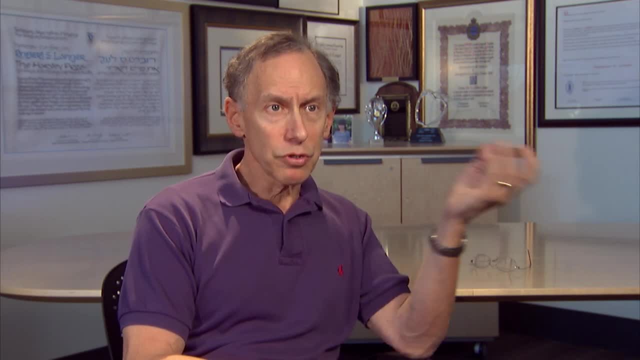 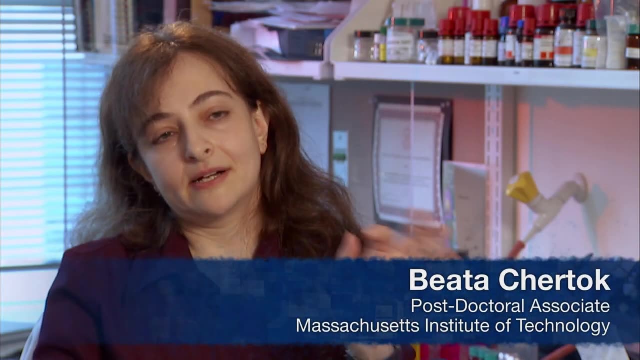 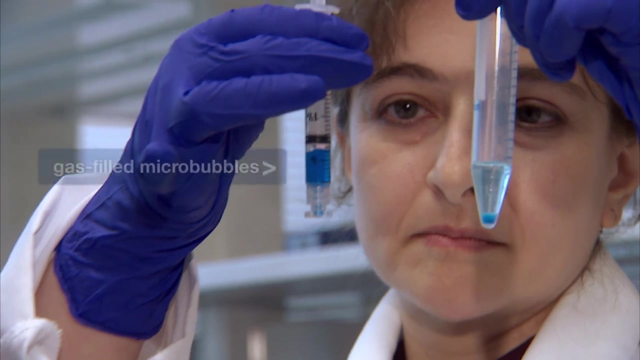 nanotechnology, where one might be able to deliver drugs right to a tumor or no other place in the body. Micro-bubbles: they are very tiny particles, micron size, And instead of being filled with liquid they're filled with gas And because of that they're visible on ultrasound and they're used to improve ultrasound diagnostics. 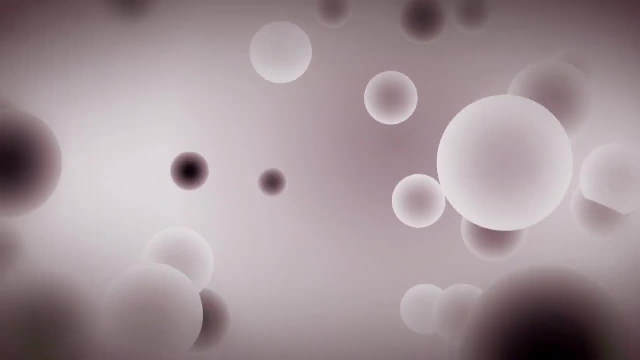 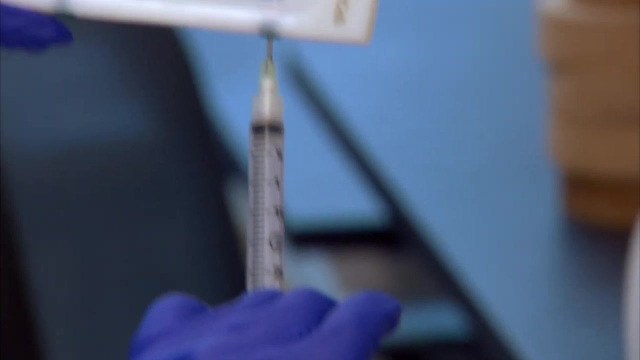 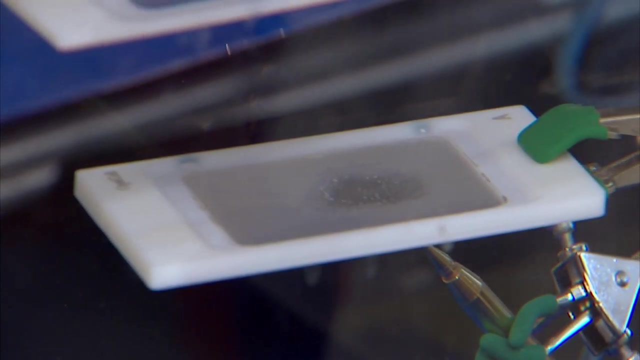 So I'm focusing on trying to incorporate drugs into these micro-bubbles. If I have those micro-bubbles loaded with drugs, I can inject them into the body. They will distribute everywhere. But then I can disrupt the micro-bubbles by an ultrasound beam and the drug will be delivered. 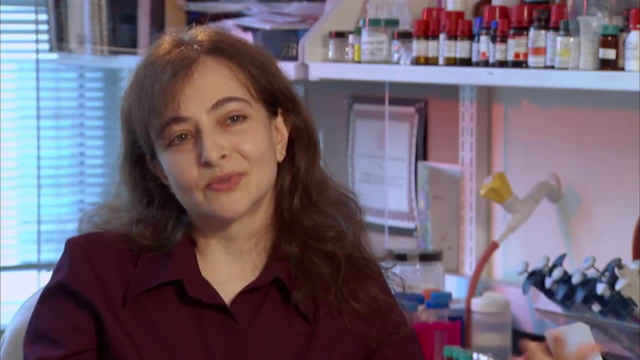 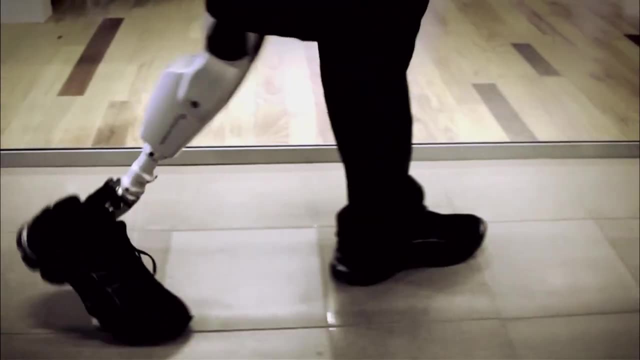 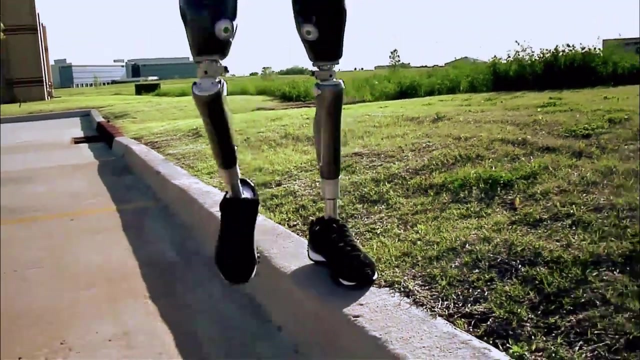 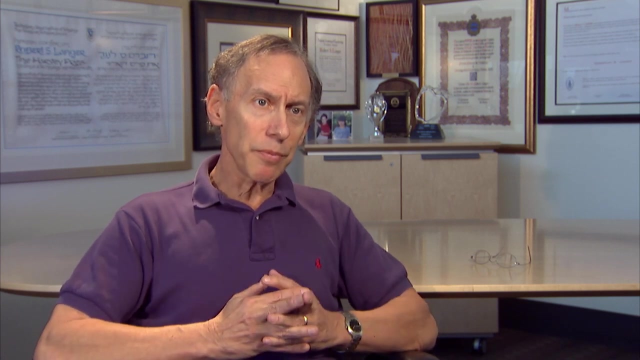 specifically where the drug is needed, And so this is the exciting engineering design that I'm working on. It's not just research that stays on demand, It's research that goes to market, goes to help people. We try to dream up things that we feel can really have a big impact, like maybe a super 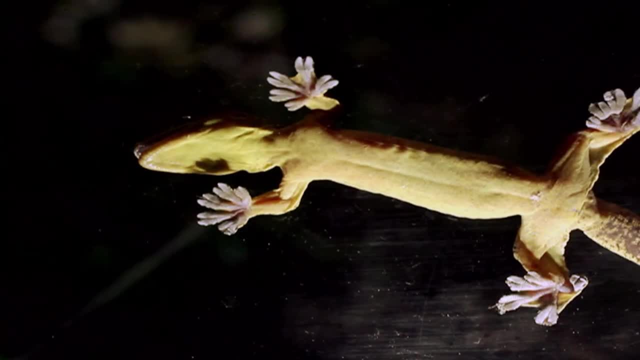 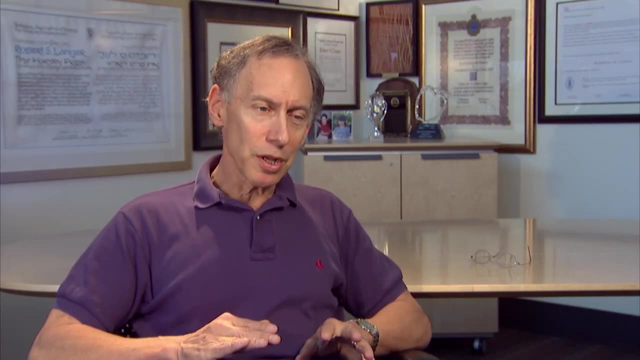 Band-Aid. We set it up to look very much like a gecko, because the gecko has enormous adhesivity on their feet, so to speak, And the Band-Aid has all these nano-protrusions from it, So there's enormous surface area. 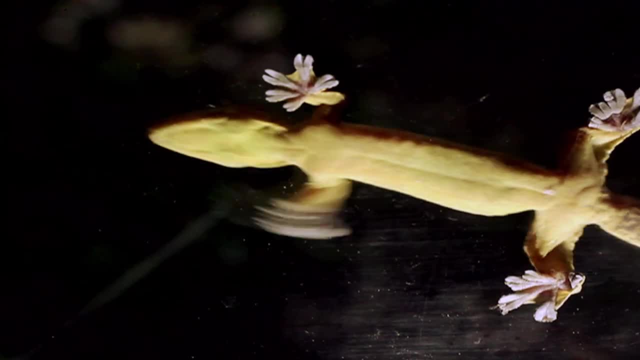 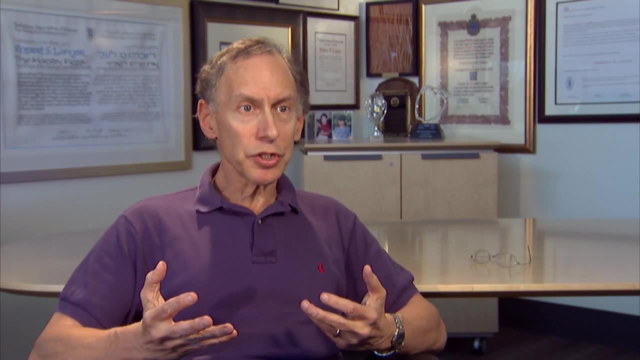 And so now we're looking at it. We're looking at it for making certain forms of surgery easier, like intestinal surgery, various different types of medical adhesive applications. A lot of times what we do is we license things to companies, or a lot of times we've started. 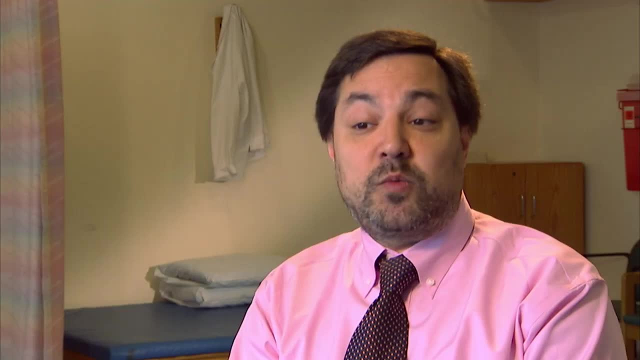 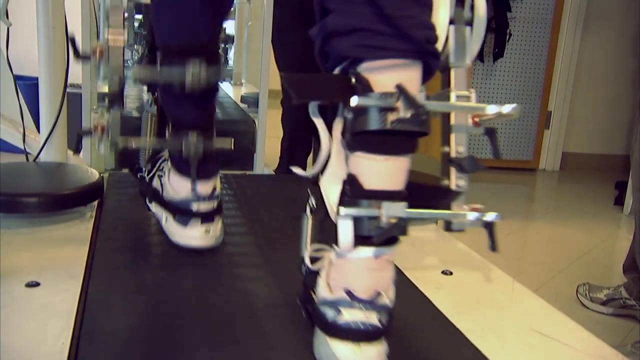 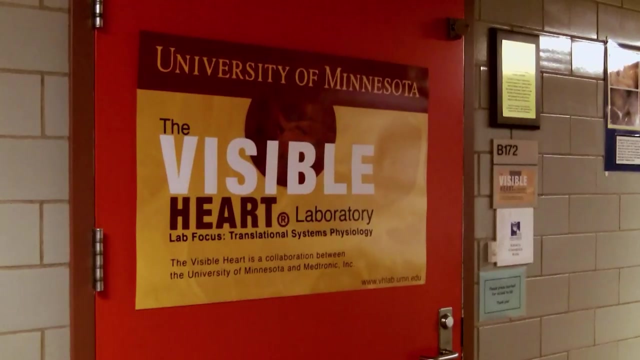 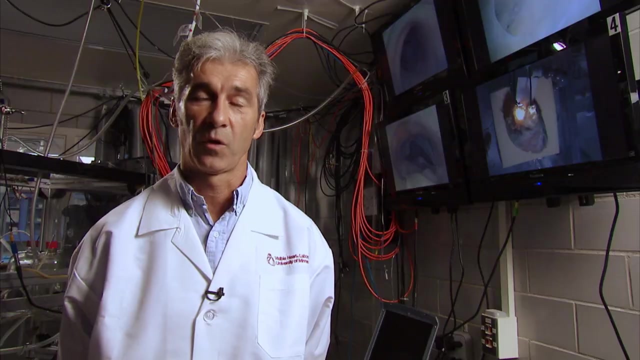 companies that create products. There is other cases in which companies are actually coming in and they're asking us to either assess their technology or redesign their technology. So we get to see cutting-edge technologies, the prototype devices. Major focus of our research is the electrical properties of both skeletal and cardiac muscle. 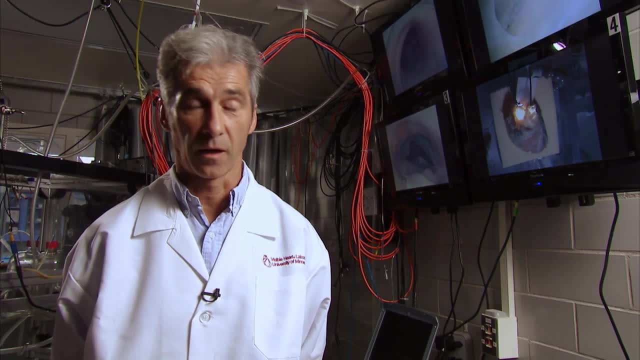 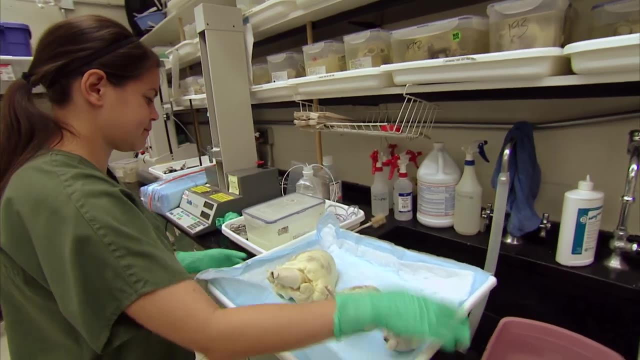 One of the things that we're doing is really novel is we're actually reanimating human hearts- And these are hearts that have been deemed non-viable for transplantation, that were gifts from the organ donors and their families to the lab, And if they have good enough function, we'll reanimate them and we'll be able to look at. 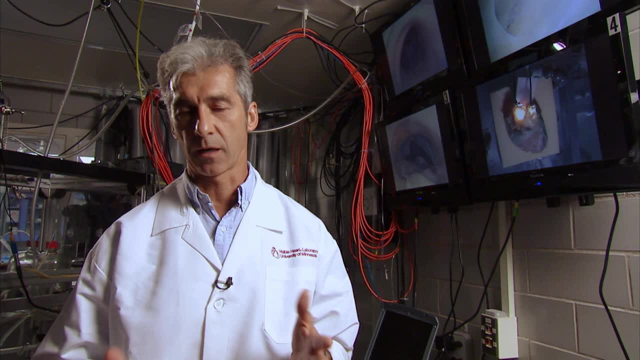 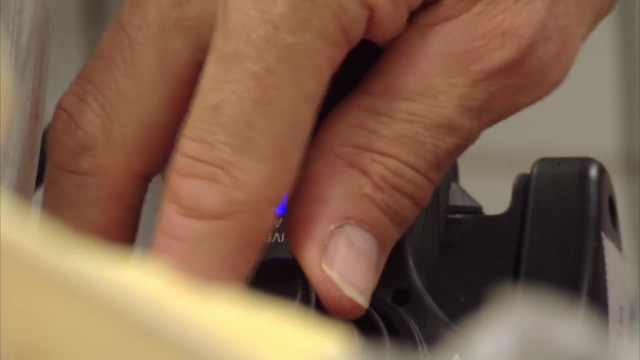 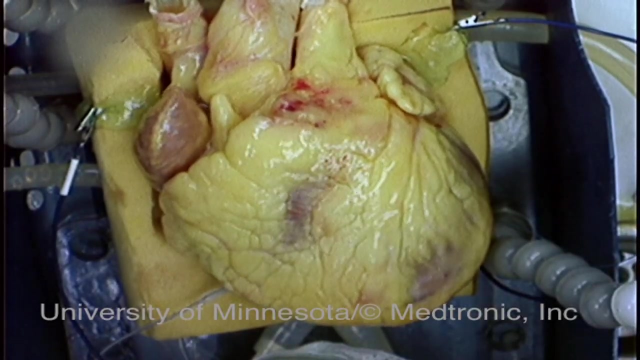 the internal anatomy while the isolated heart is functioning And just like a heart transplant, you have four to six hours Before you need to reanimate that heart. We'll get it to beat on its own in a native rhythm and then we can put cameras inside. 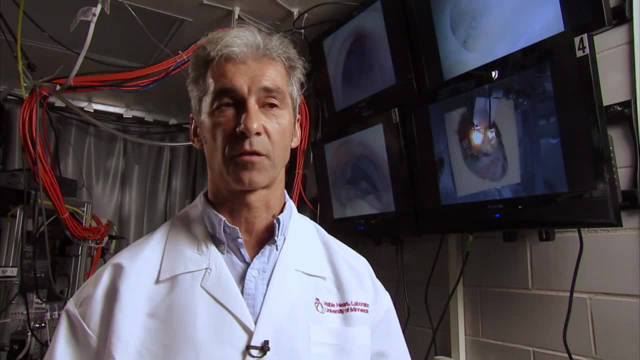 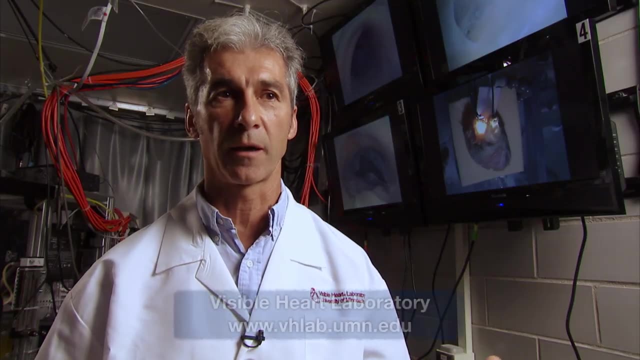 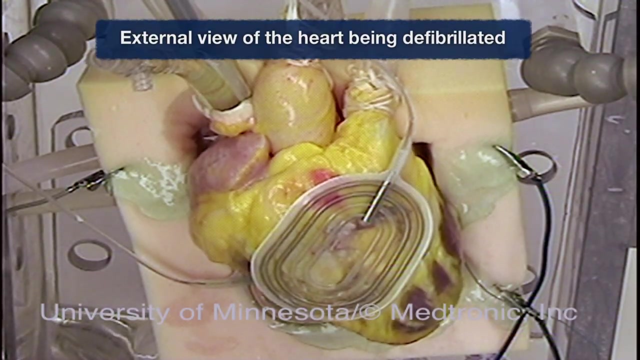 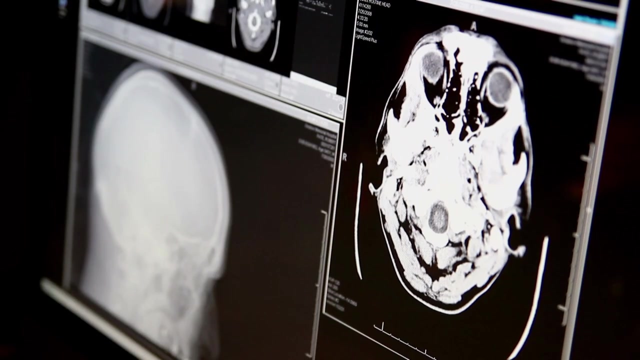 and visualize any of the functional anatomy, really study this device, tissue, interface of new pacing systems or leads. We actually have a whole free access website that anybody can go online and see the functional anatomy from these human hearts. Biomedical engineering is not just a field for engineers, but also there's a bio side. 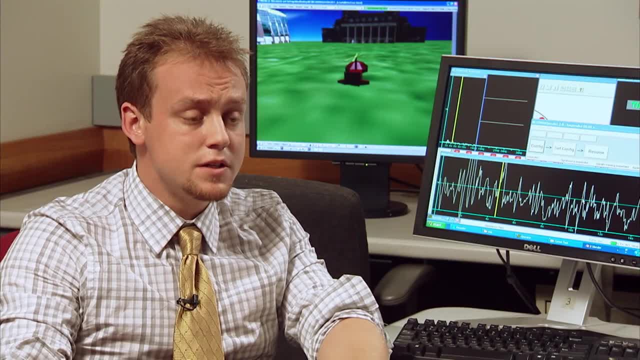 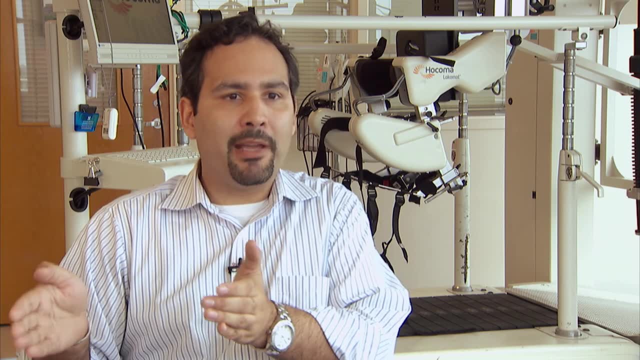 The physicians who are working in the clinics every day are going to see what the problems are, And the engineers may have already solved those problems and not even know they're there. Patients get whatever the engineers make. engineers make whatever they think the patients need. 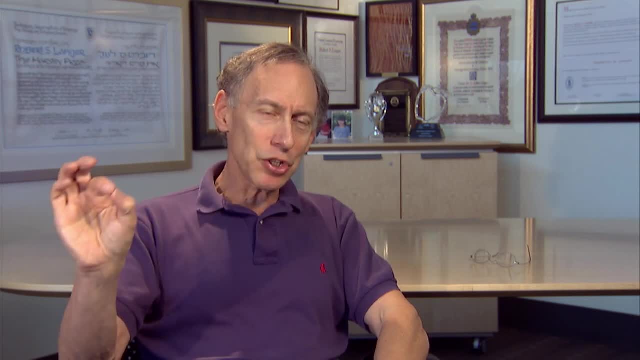 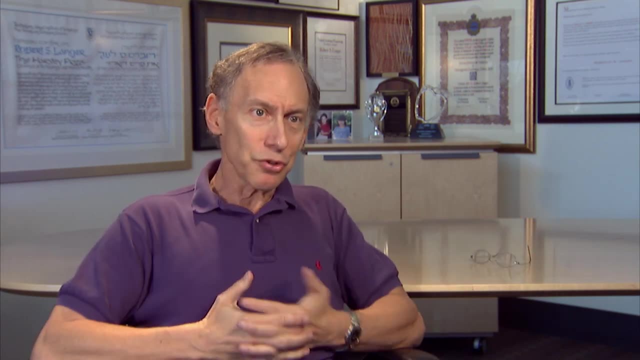 The way I look at it is: the physicians are able to ask great questions and the engineers are able to come up with great answers, But if you just have one and not the other, you don't solve them because you don't even know what to ask or don't know how to answer it. 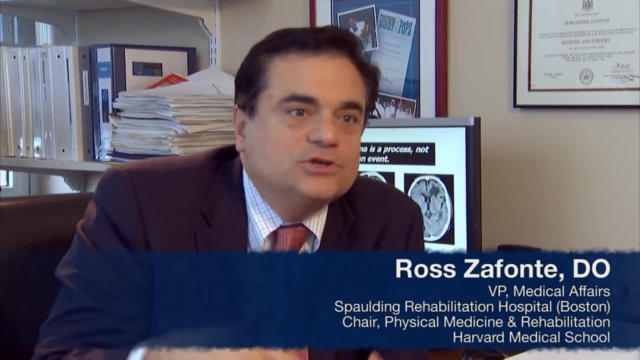 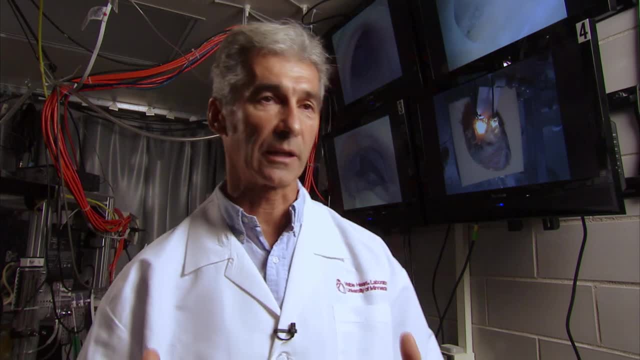 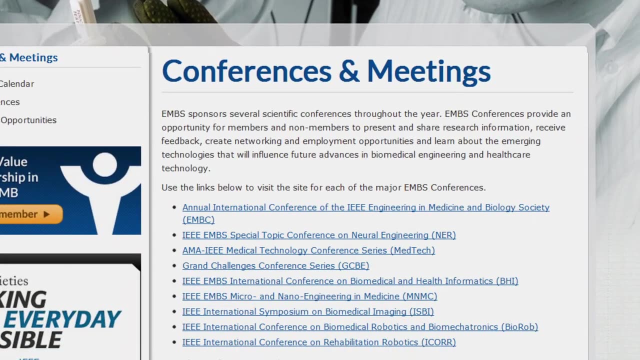 So we like to establish things as an iterative loop, as a loop where people are going back from the laboratory to the clinic and then back to the lab again refining our questions. So it really helps to keep everybody's research very relevant. I initially joined the Engineering and Medicine Biology Society to be able to connect with 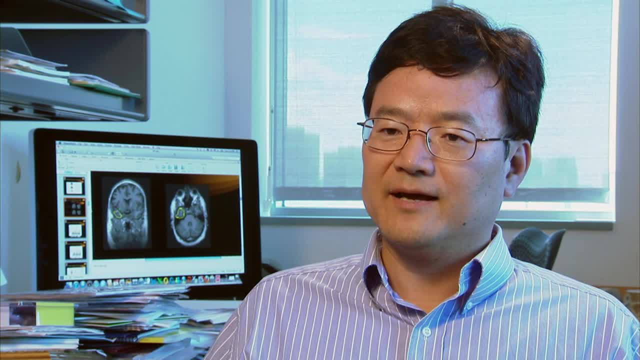 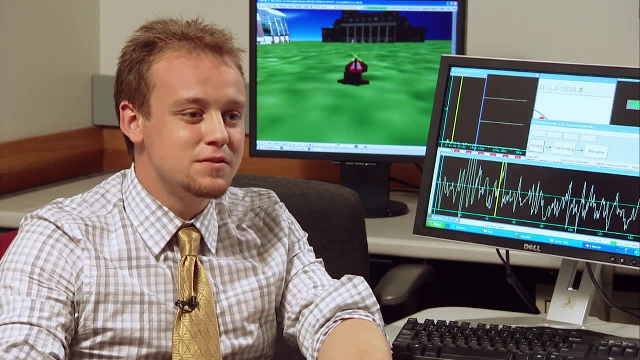 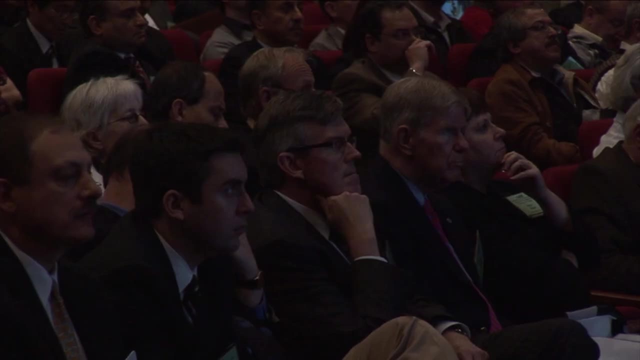 other like-minded people. That's where I feel that I learned what exciting science is going on in the field. You can kind of get this teleportation right to the cutting edge of a field and be part of that discussion. For physicians, being a part of the MBS provides an opportunity to be exposed to new technologies. 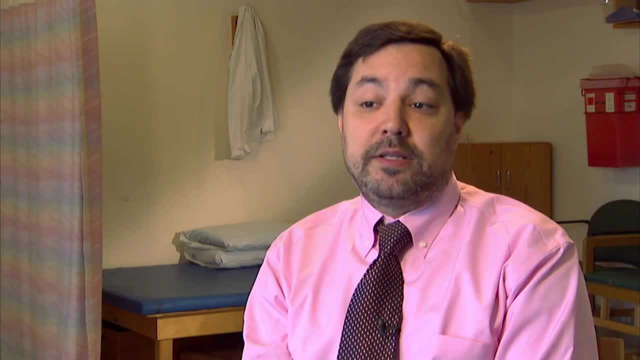 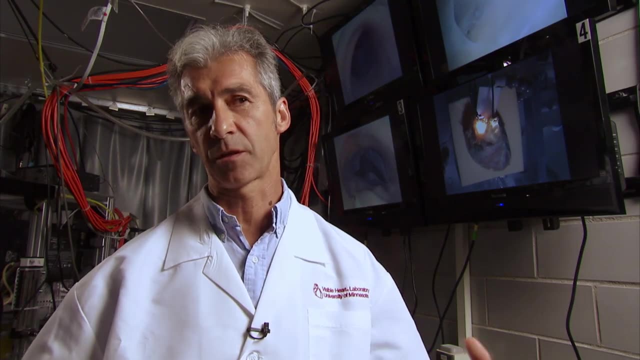 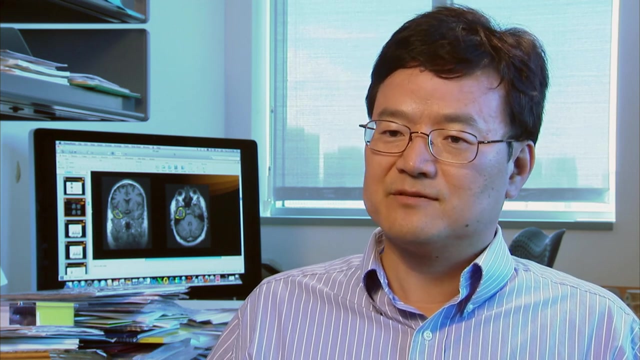 to provide feedback about the way we're developing this technology within the engineering field, And I think it's this partnering with all these different disciplines from these different careers that really is essential to move the field forward. I feel I belong to part of an important professional network which is making a big impact to the 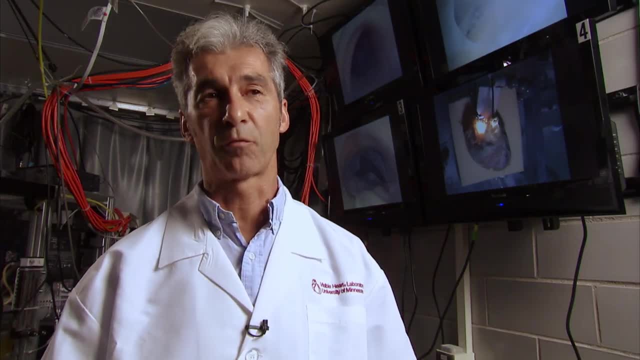 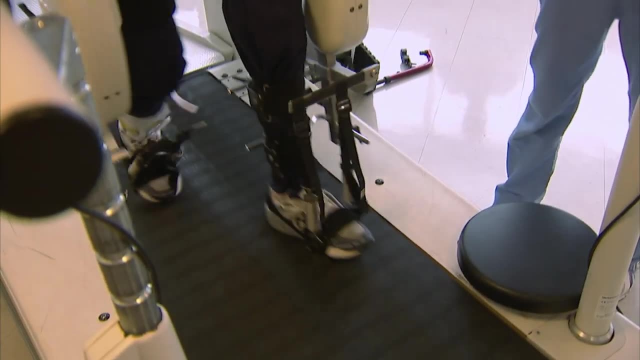 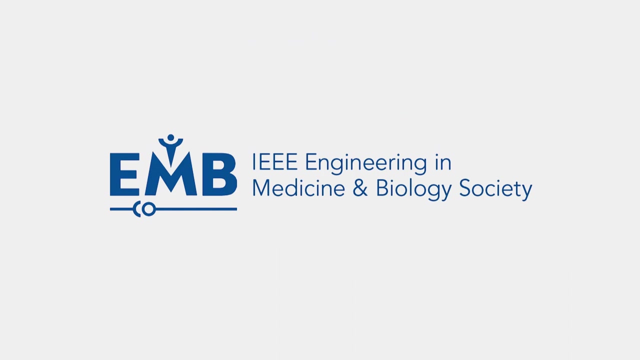 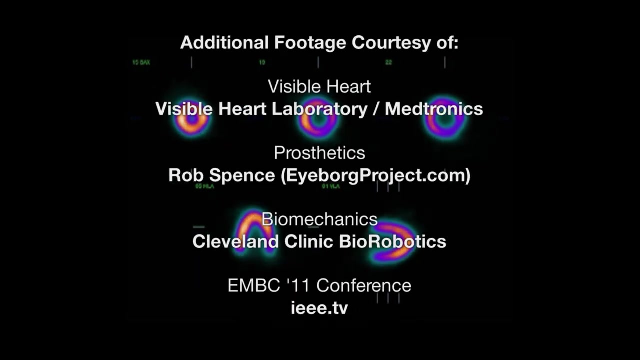 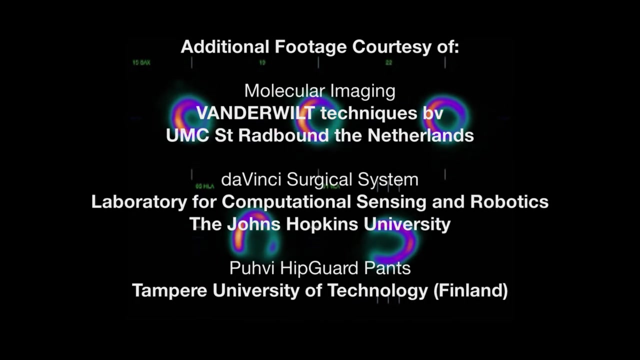 society. It's only exciting if research actually makes it off the bench top and helps people. You know, it's just. it's exciting to make a difference. Is it a great opportunity for our community? It is a great opportunity. Thank you for your attention. 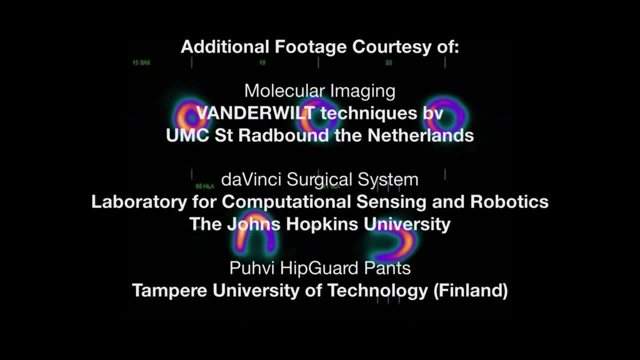 Thank you for learning, Thank you for being here.